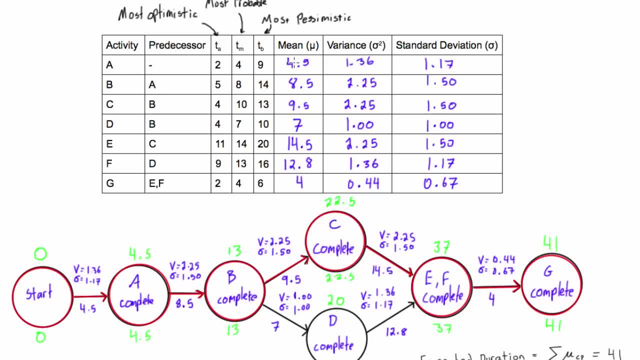 the expected duration of any individual activity. for example, activity A. well, its expected duration was 4.5 days, but we know that you know, it could be as bad as 9 days, or it could be as good as 2 days. right, It's somewhere in this range. So what we want to do is we 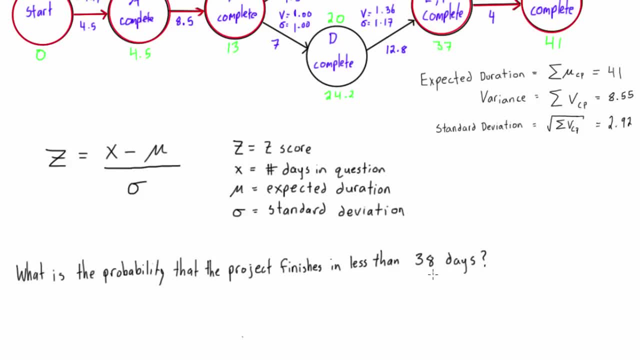 want to figure out. yeah, here's what we want to do. So we're going to find out the probability that our project will finish in less than 38 days. So all we do is we calculate our z-score and our z-score uses. here let's fill in our equation. here Let's maybe change. 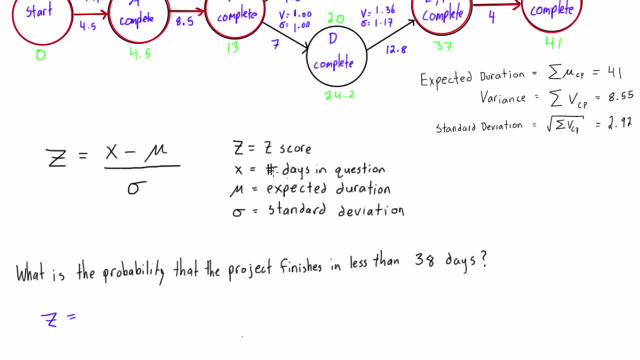 the color. So we have z will be equal to x. This is the number of days in question, so that will be 38 in this case, 38 minus mu, which is our expected duration. so that's 38 minus 41, and over our project standard deviation, which was 2.92.. 2.92.. So if you 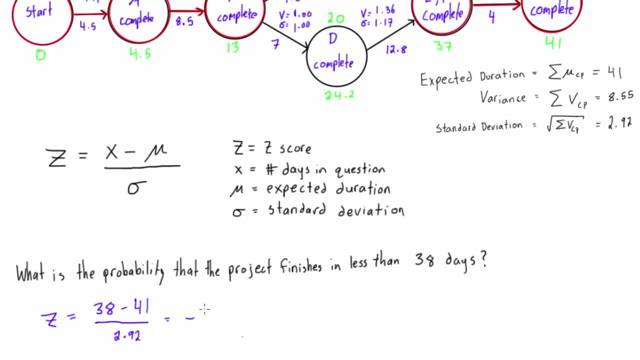 just punch that in your calculator, you actually get a z-score that is negative, 1.03.. Okay, so what we do with the z-score? this z-score can lead us to a probability, So we have to go to a z-score table. It's in the back of any statistics book, or if you just Google. 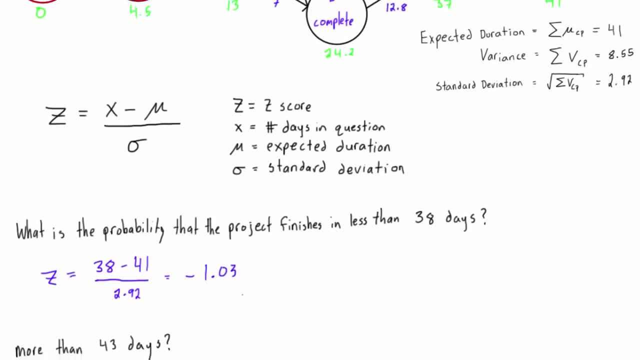 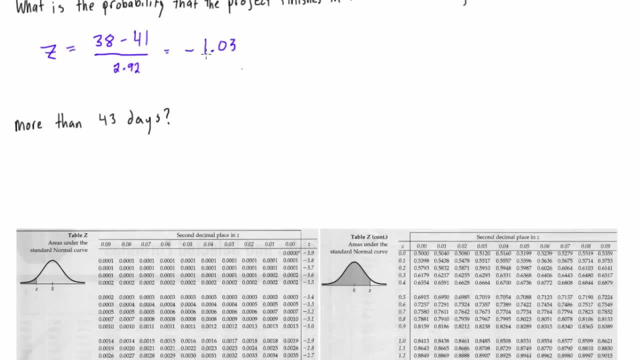 image search z-score table, you'll come up with an endless supply of them. So I found a z-score table for us to use down here. Let's take a look at them. So, first of all, we're looking for a z-score of negative 1.03.. What we look at down here is there's two possible 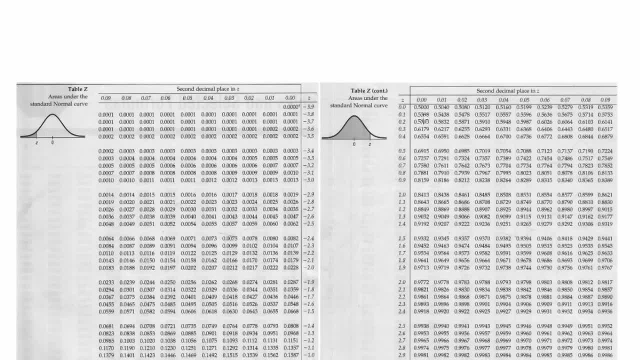 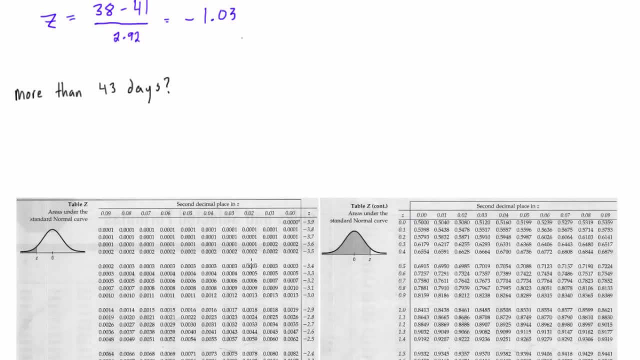 z-score tables we can use or z-score tables, One where our z-score will be negative and one where our z-score will be positive. So we have to locate our number, our z-score, and it will return one of these probabilities that's floating in the middle of the table. 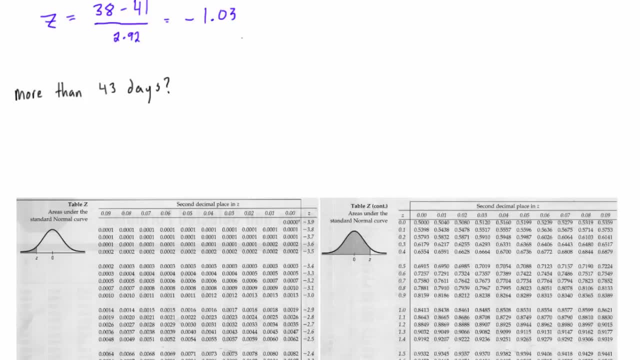 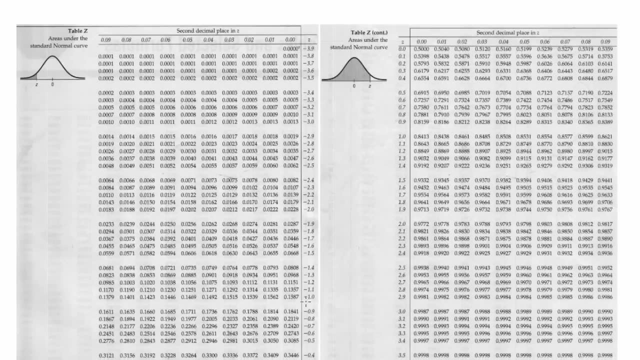 So our z-score is negative 1.03.. So it will be on the negative table. We come down here First, we'll locate negative 1.. We have to go a little bit further than that. So we have negative 1, and it was 0.03,. so we come up here: and it was 0.03, right? So negative 1.03.. 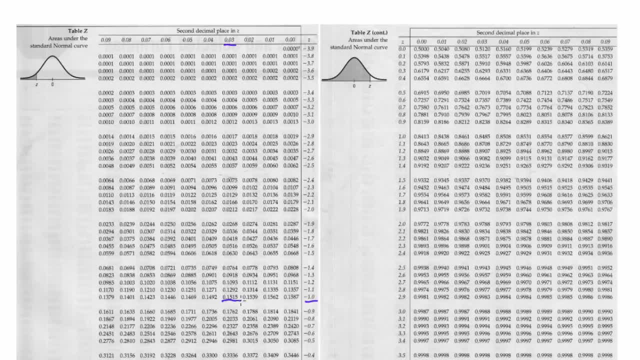 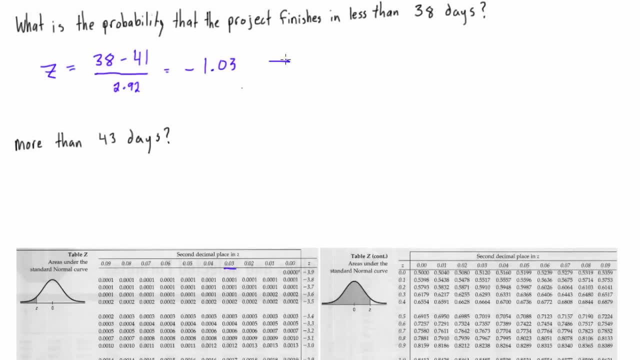 We find out where those two match and we're getting this value here of 0.1515.. So first of all, let's write that down. So this is giving us this probability. Probability of z. this particular z-score is equal to 0.1515.. Now what that means is that the probability of landing in 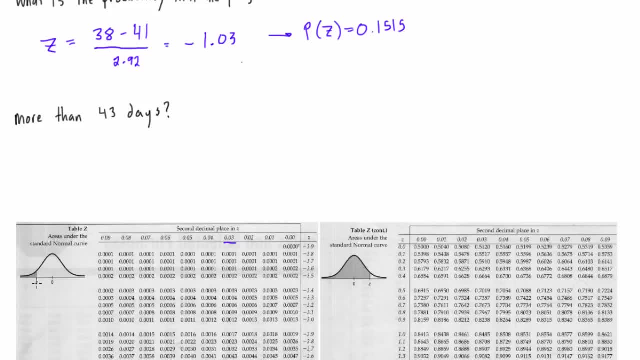 this shaded region here on your bell curve is 15.15%. But what does that even mean? So let's look at this first of all. Well, your bell curve here will be centered over your mean, so that's 41. And this x value here. 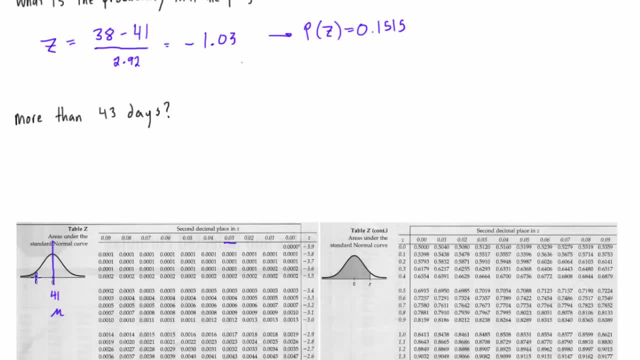 so we can even write that. so that's mean, And this x value here, well, that's 38. That's the day that we're looking at, And this is actually why we're getting a negative value, because we're looking at 38. If we were looking at a number that was larger than 41, we'd be getting a positive. 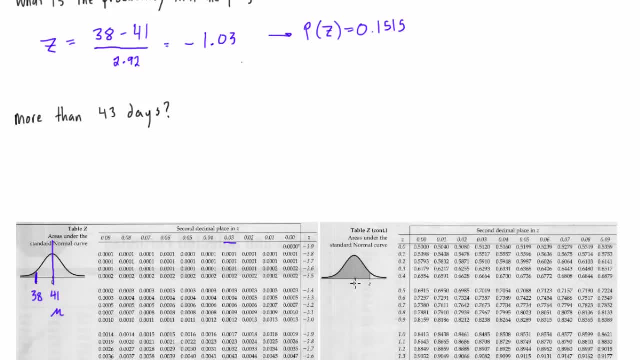 value, hence that this x is on the positive side of that would be 41,, where here it's on the smaller side. All right, And this is our x value. So this is saying that this is all. the z-score table will always give you the probability of. 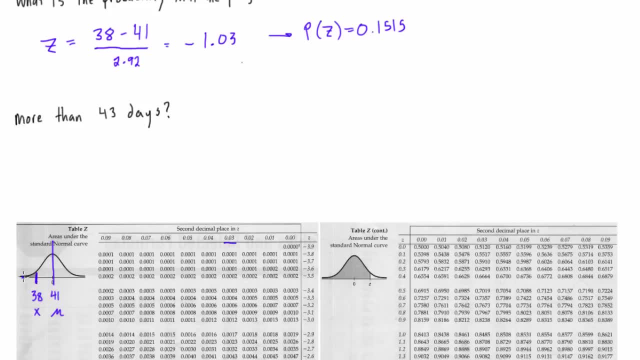 landing in a shaded region, no matter which one you're using. So now we're saying we have a 15% chance of landing here in the shaded region, And this shaded region is anything that's less than 38.. So the original question was: what is the probability that the project finishes in less? 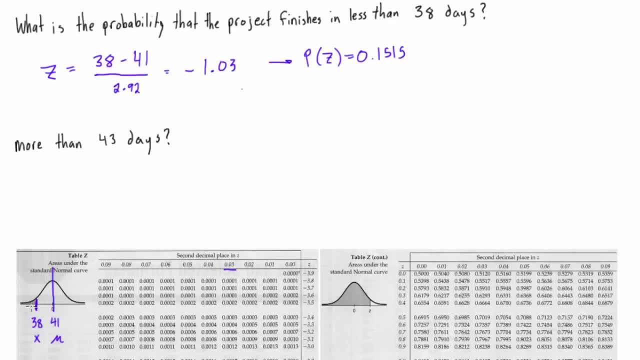 than 38 days. Well, that's this probability, right? Anything. this could be 37,, 36, and it just trails off basically down to nothing. So, the probability that we finish in less than 38 days, we're going to get a probability of actually 15.15%. All right, Now let's look at something. 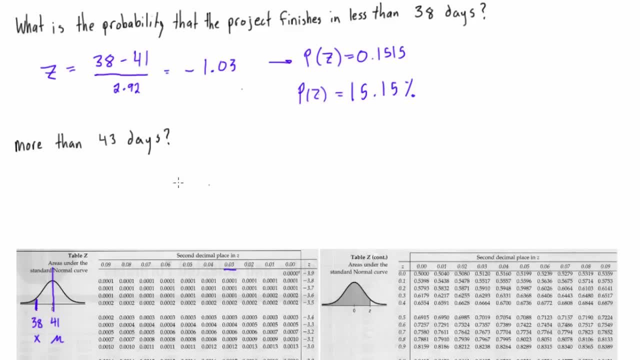 let's look at the other example, where we're going to be more than 48 days. So we will change this slightly. So our z-score now will be: z is equal to 43, 43 minus 41 over our standard deviation, which was 2.92.. And if you just punch that in your calculator, we will be getting a value of 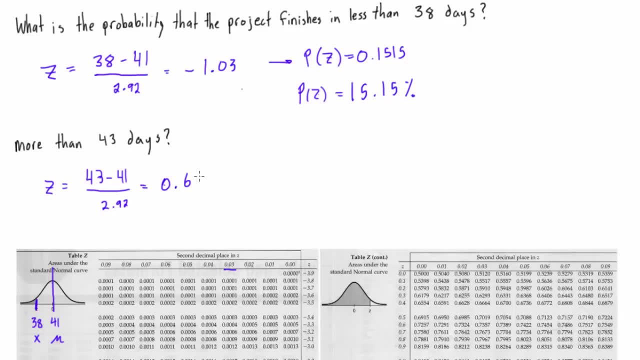 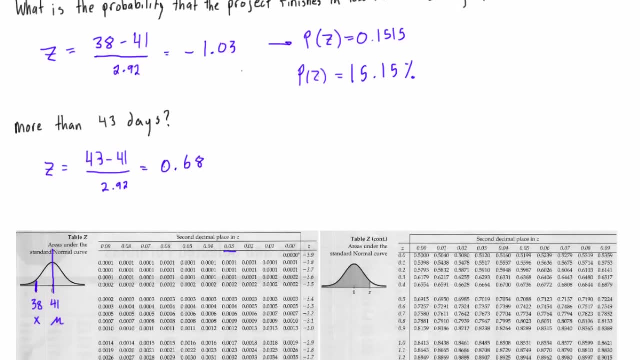 0.6849, 6849.. And let's actually just round that to 68, 0.68.. That's good enough, All right. So when you're we're going to come down into our z-score tables, we have a positive value, So. 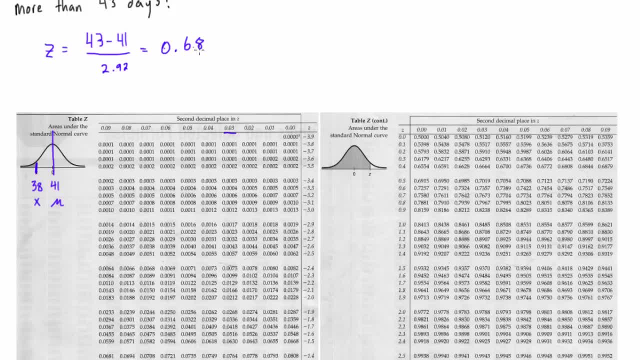 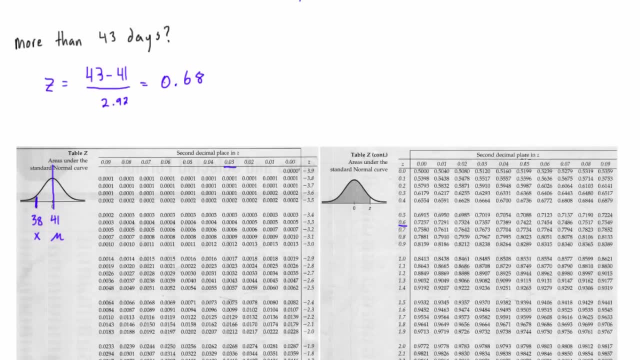 we're not using the negative values. We need to find the positive value, And so 0.68, let's come down, We'll be. we'll actually be up close to the top here. So we have 0.6 and 0.8 will be right. 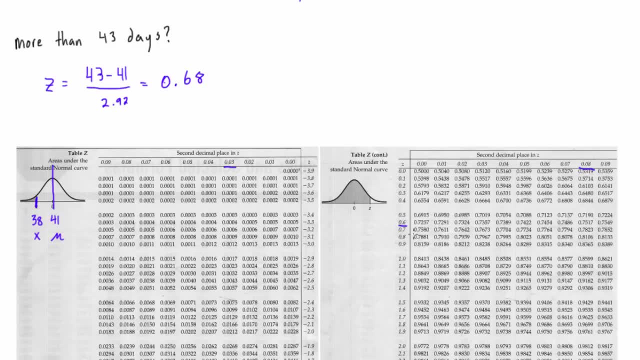 here. So that would give us 0.68.. And then we meet with our z-score here. So we're going to find where those two meet and we get this value in here. So then we're saying that this is giving us the probability of being less than the z-score actually is going to be 0.7517.. 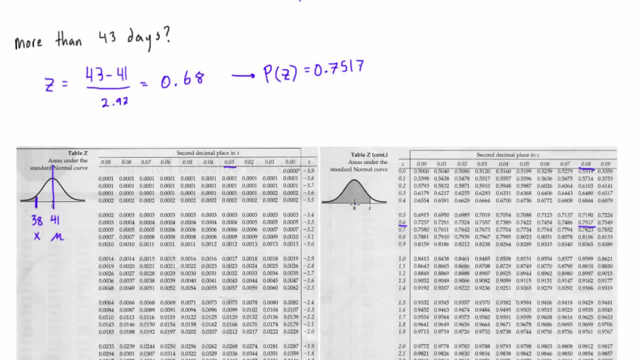 All right, So, but notice how I said that. I said that's the probability of being less than, and that's because, again, we're situating our mean here at 41.. We're setting up our x value here at 43. And, again, this was our mean, this is our x And this is saying the probability. 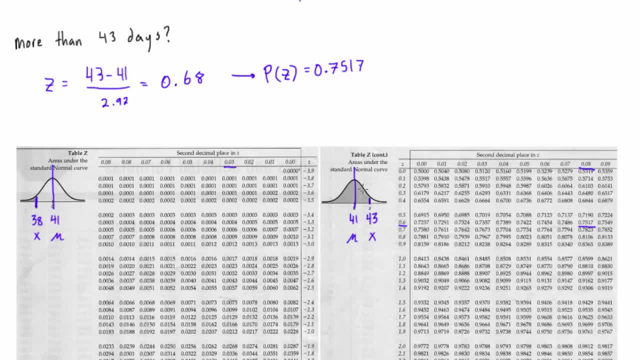 this z-score and this probability for that z-score, the probability of being less than so in this shaded region, so anything less than 43, that would include 42,, 41,, 40,, 39,, et cetera. 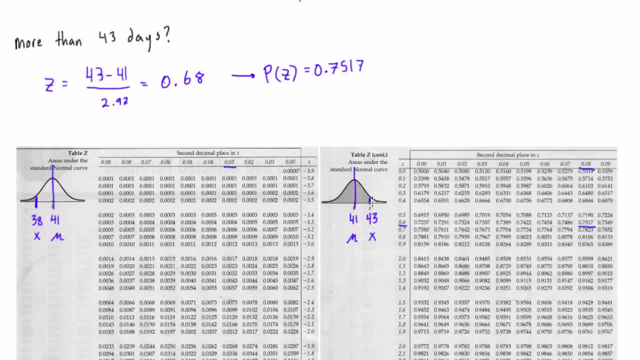 That probability is 75% probability, but we're looking at the probability. We want to find the probability here. for blue That's a greater than So. everything under this curve is a hundred percent of the probability, or you can think of it as one. So what we have here, we're actually